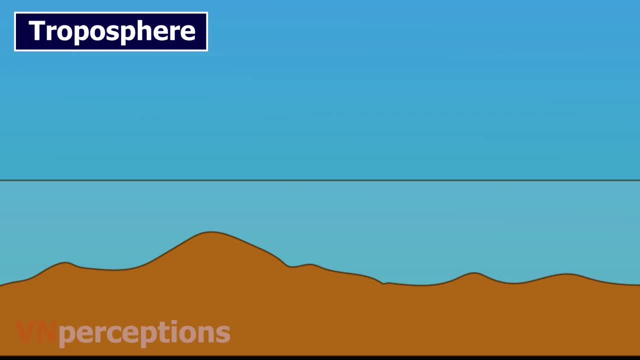 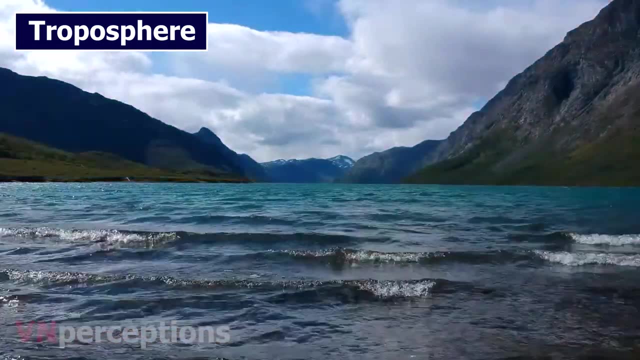 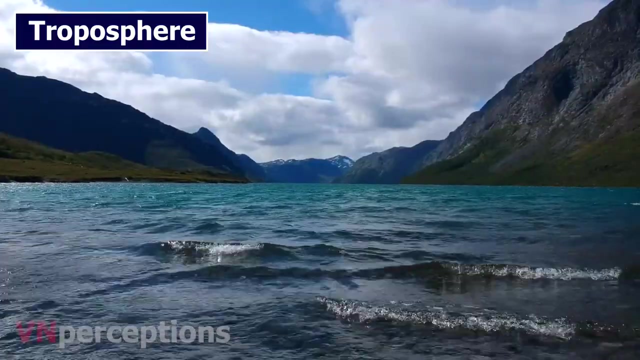 that is, about 75 to 80 percent of the atmosphere is in the troposphere. Most of the types of clouds are found in the troposphere and almost all weather occurs within this layer. The troposphere is by and far the wettest layer of the atmosphere. 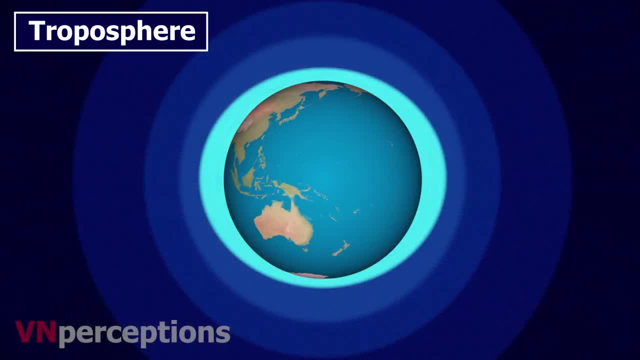 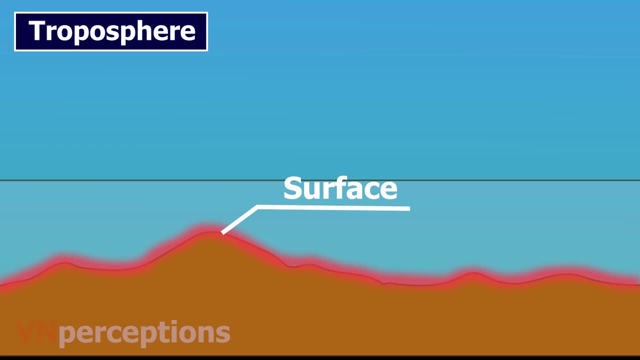 and all the layers above contain very little moisture. The bottom of the troposphere is the earth's surface. The height of the top of the troposphere varies with latitude. Its average is 13 kilometers and extends roughly to a height of 8 kilometers near the poles. 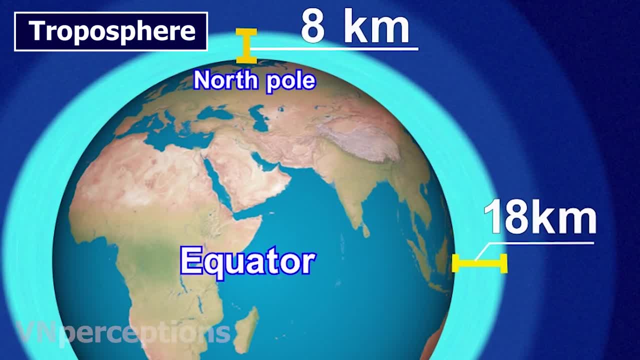 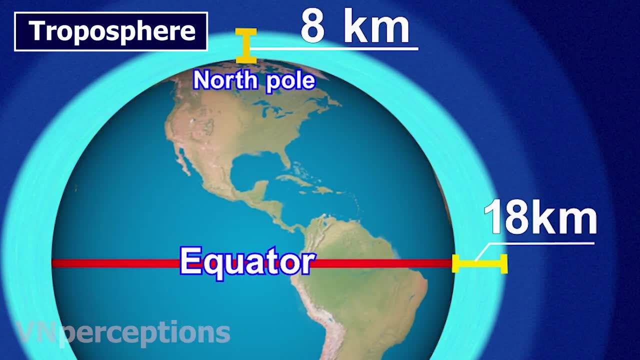 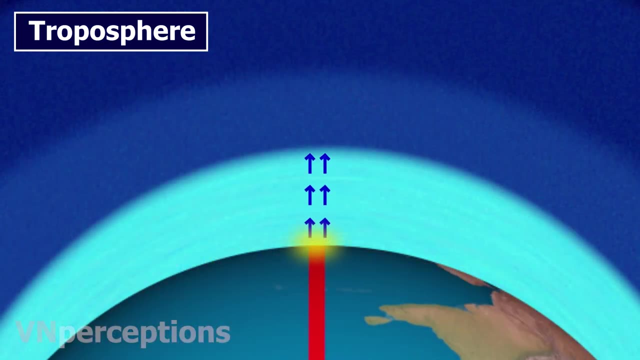 and about 18 kilometers at the equator. So what do we understand? It is lowest over the poles and highest at the equator. The thickness of the troposphere is greatest at the equator because heat is transported to great heights by strong convectional currents, that is. 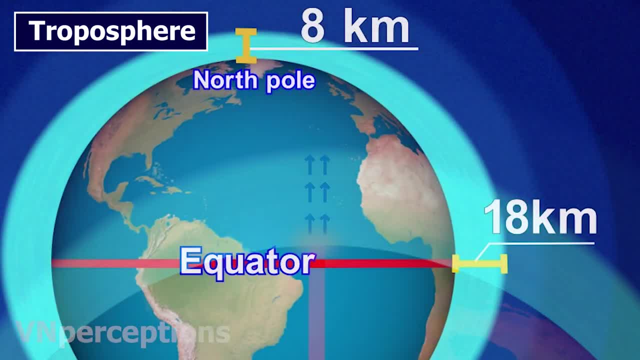 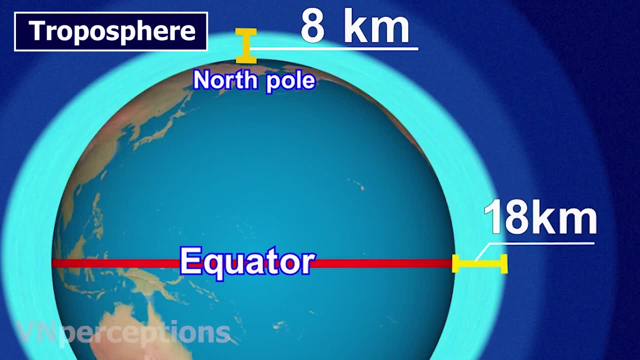 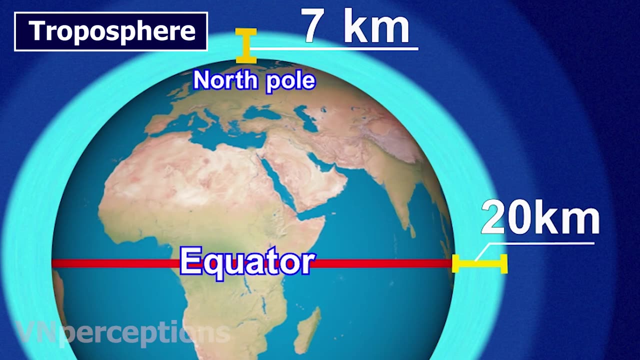 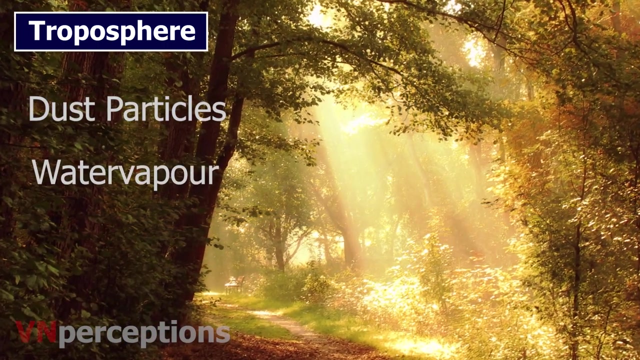 vertical currents. here. The height also varies by season: It is lower in winter and higher in summer. It can be as high as 20 kilometers near the equator and as low as 7 kilometers over the pole in winters. Now, this layer contains dust particles, water vapor, storm clouds. 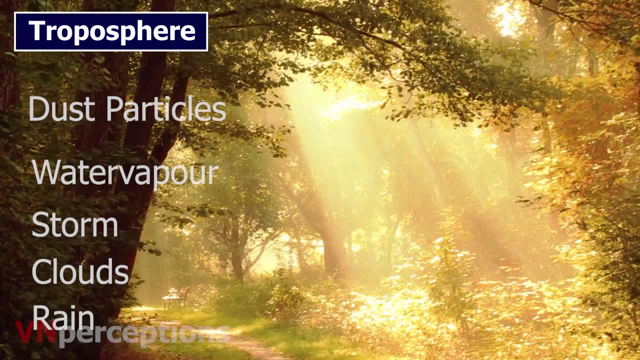 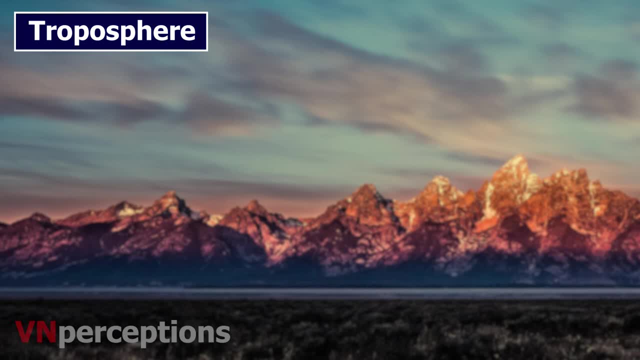 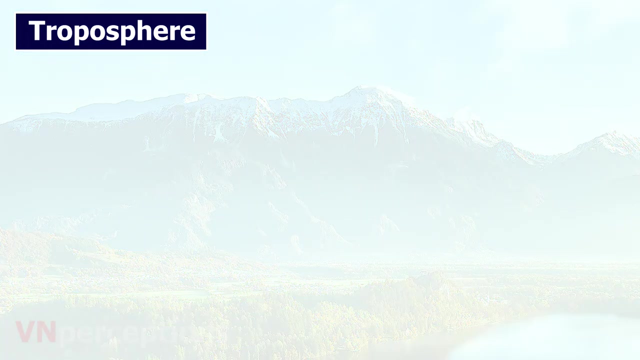 and rain. All changes in climate and weather takes place in this layer. The temperature in this layer decreases at the rate of 1 degree for every 165 meters of height. That is why the peaks of tall mountains can be snow covered even in the summertime. This is the most important layer of 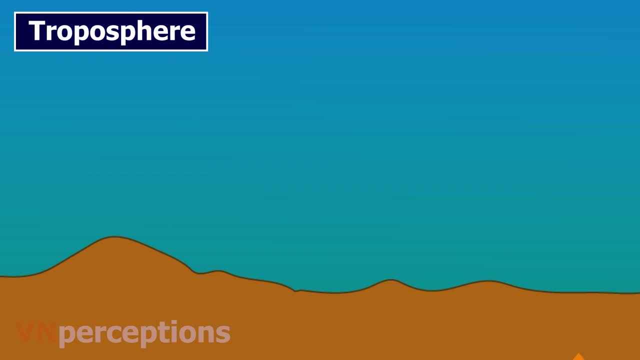 all biological activities In this layer. the temperature of the top of the troposphere is decreased with height. The reason is the density of air decreases. It means the density of air is high near the ground and as we go to higher altitudes the density of air decreases. So there 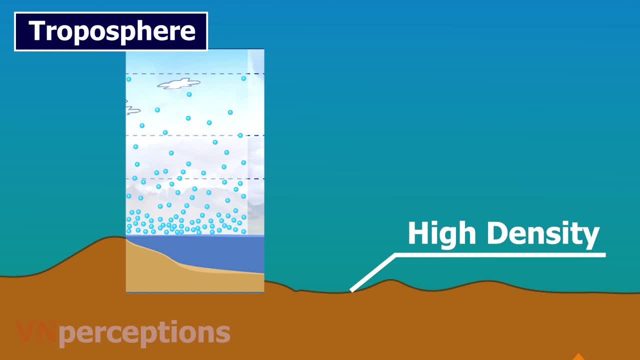 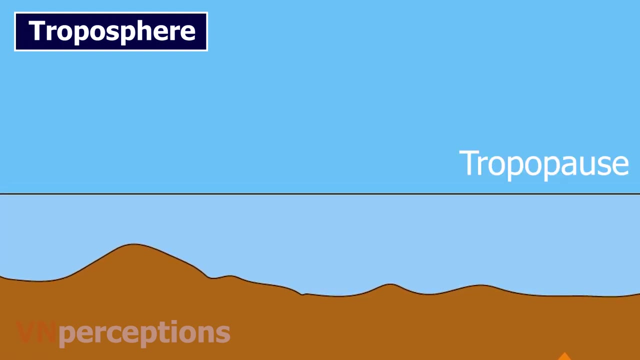 are less air particles and the heat absorbing capacity of the air decreases, And that is why, when you go to higher altitudes, it is less air particles and the heat absorbing capacity of the air is high. The zone separating the troposphere from stratosphere is known as tropopause, The 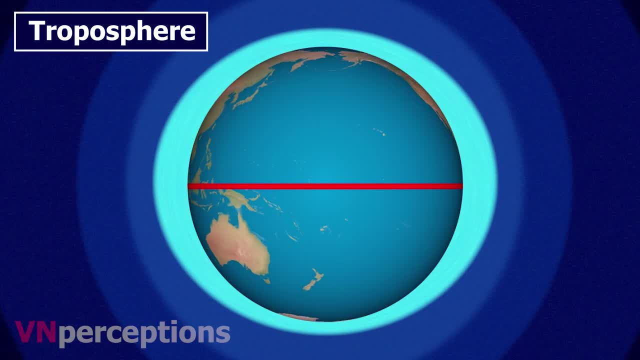 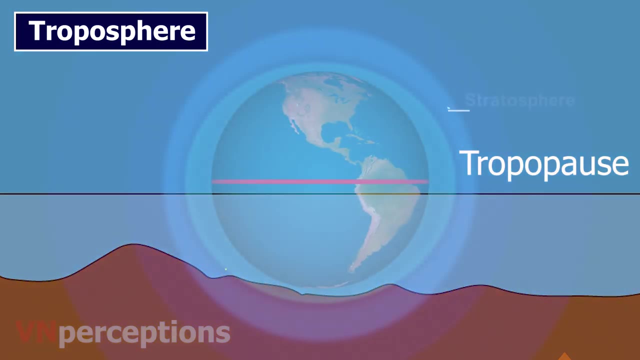 air temperature at the tropopause is about minus 80 degrees Celsius over the equator and about minus 45 degrees Celsius over the poles. The temperature here is nearly constant, and hence it is called tropopause. Then comes the stratosphere. The stratosphere is found above the tropopause and on 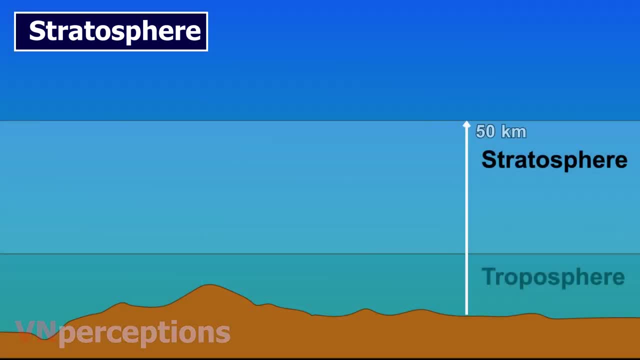 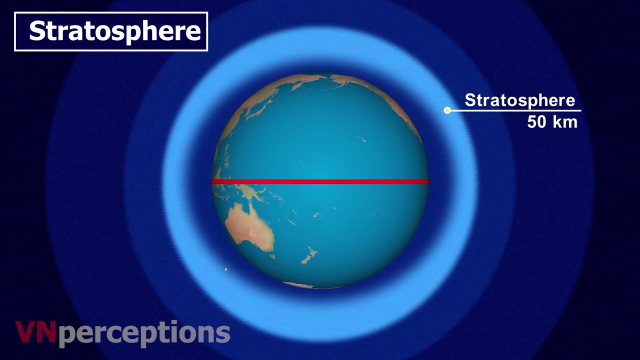 and extends up to a height of 50 kilometers. The bottom of the stratosphere is around 10 kilometers above the ground at mid-latitude. The top of the stratosphere occurs at an altitude of 50 kilometers. The height of the bottom of the stratosphere varies with latitude and with. 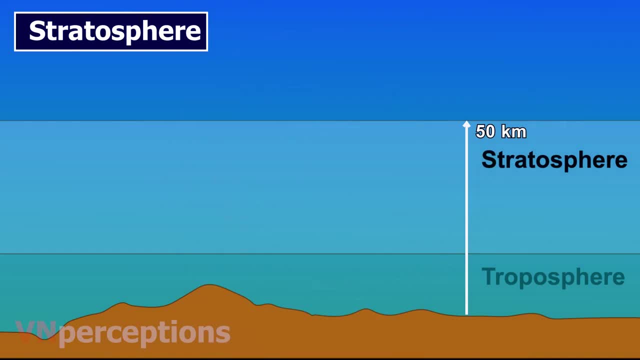 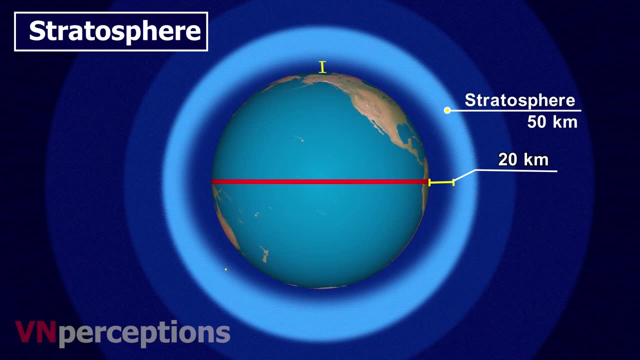 the seasons, The lower boundary of the stratosphere can be as high as 20 kilometers near the equator and as low as 7 kilometers at the poles in winter. The lower boundary of the stratosphere is called the tropopause. The upper boundary is called stratopause, One important 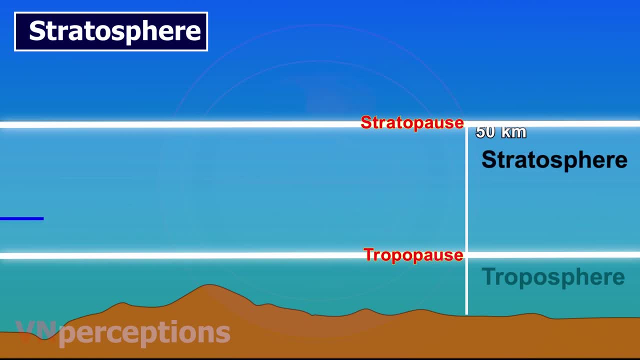 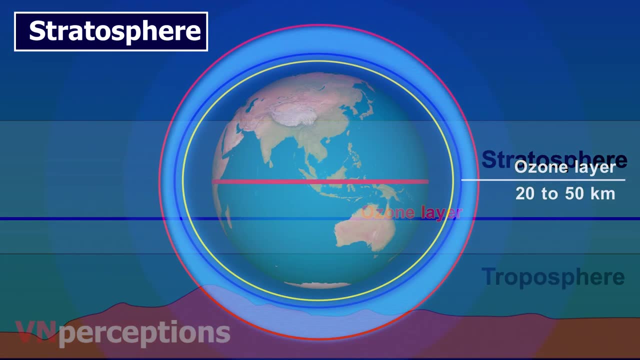 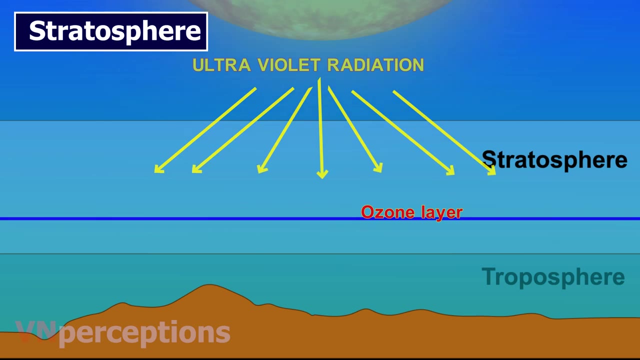 feature of the stratosphere is that it contains the ozone layer. It lies between altitude 20 to 50 kilometers. It heats this layer as it absorbs energy from incoming ultraviolet radiation from the sun. Temperatures rise as one moves upward through the stratosphere. 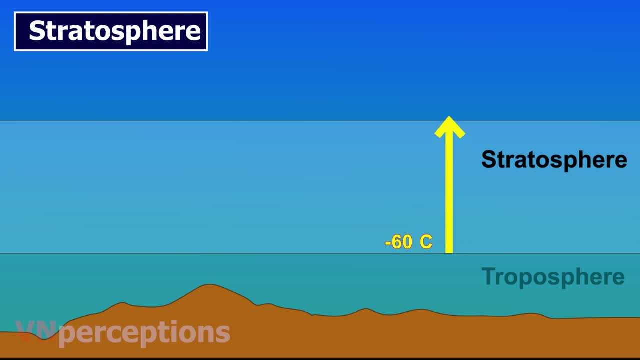 Temperature rises from minus 60 degrees Celsius at the base to zero degrees Celsius at the stratopause. This is exactly the opposite of the behavior in the troposphere in which we label, where temperature drops with increasing altitude Because of this temperature stratification. 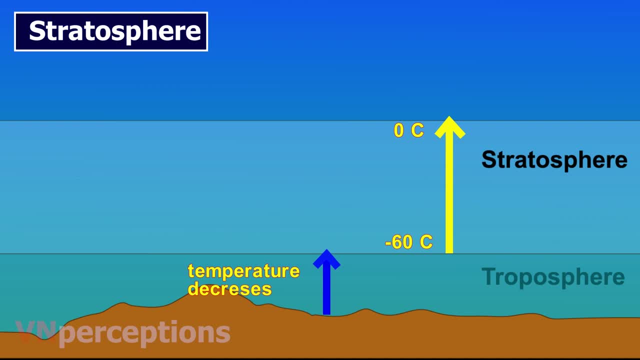 that is because of this temperature layers there is little convection and mixing in the stratosphere, So the layers of air there are quite stable. Commercial jet aircraft fly in the lower stratosphere. This is to avoid turbulence, which is very 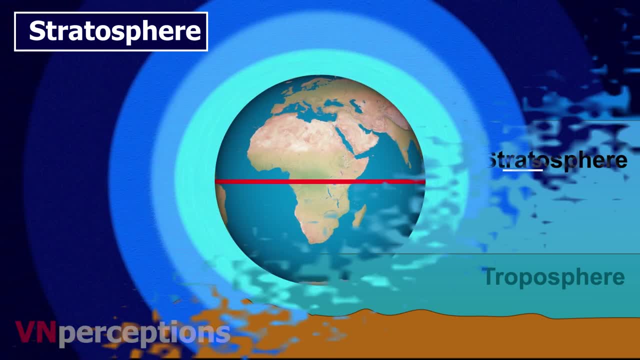 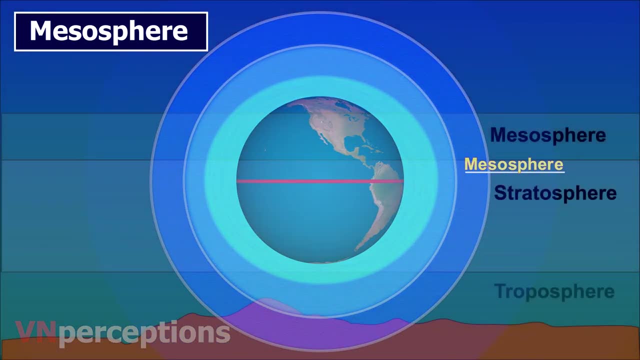 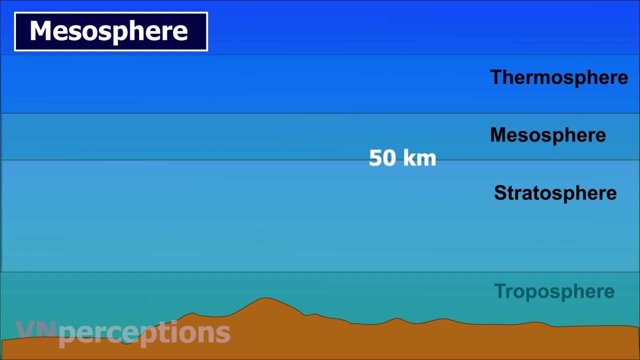 common in turbo star troposphere. Next comes mesosphere. The mesosphere is a layer of earth's atmosphere. It is directly above stratosphere and below thermosphere. It extends from about 50 to 85 kilometers above our planet. Temperature decreases with height throughout the mesosphere. 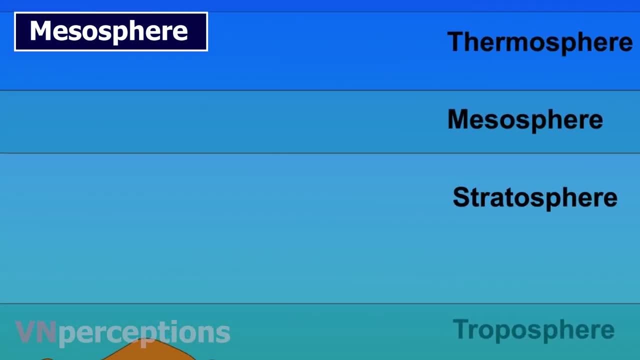 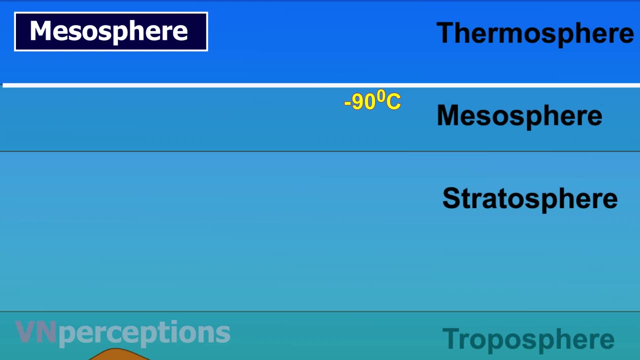 The coldest temperatures in earth's atmosphere, that is, about minus 90 degree celsius, are found near the top of this layer, The boundary between the mesosphere and the thermosphere above it is called the mesopause. At the bottom of the mesosphere is the stratopause. that is the boundary. 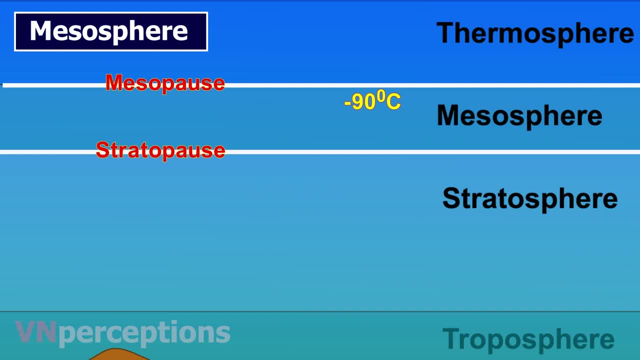 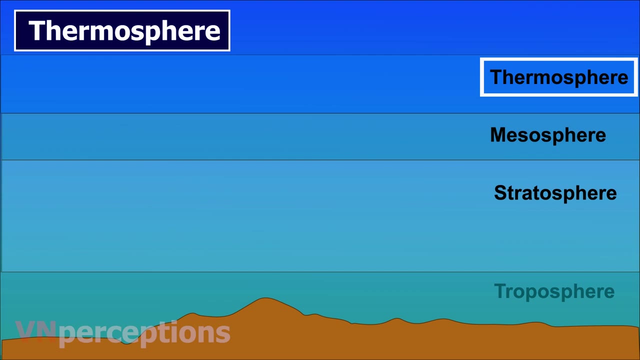 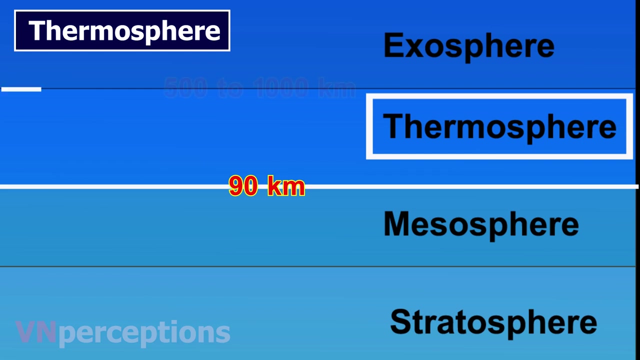 between the mesosphere and the stratosphere below The mesosphere is difficult to study, so less is known about this layer. Then comes the thermosphere. The thermosphere is directly above the mesosphere and below the exosphere. It extends from about 90 kilometers to between 500 to 1000 kilometers above our planet. 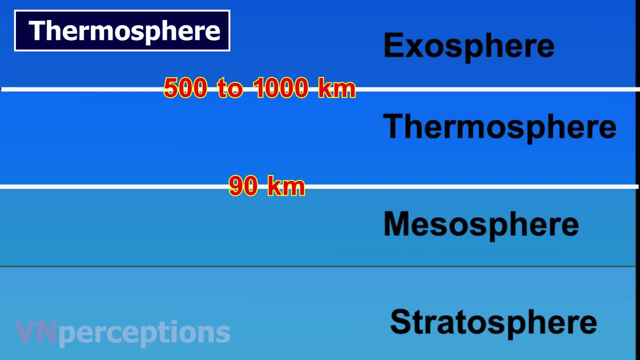 Temperatures climb sharply in the lower thermosphere, then level off and hold fairly steady with the increasing altitude above their height. Solar activity strongly influences temperature in the thermosphere. The thermosphere is typically about 200 degree celsius hotter in the daytime than at night. 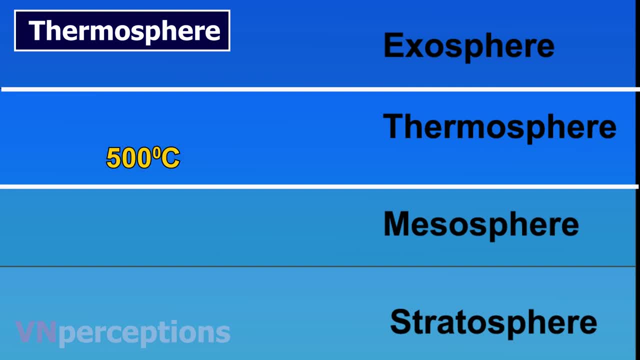 and roughly 500 degree celsius hotter when the sun is very active than at other times. Temperatures in the upper thermosphere can range from about 500 degree Celsius to 2000 degree Celsius or higher. The boundary between the thermosphere and the exosphere above is called thermopause. 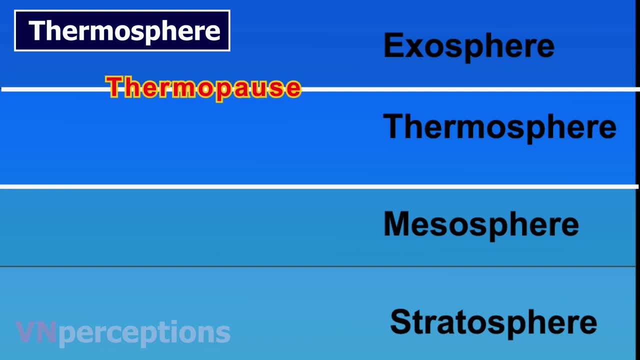 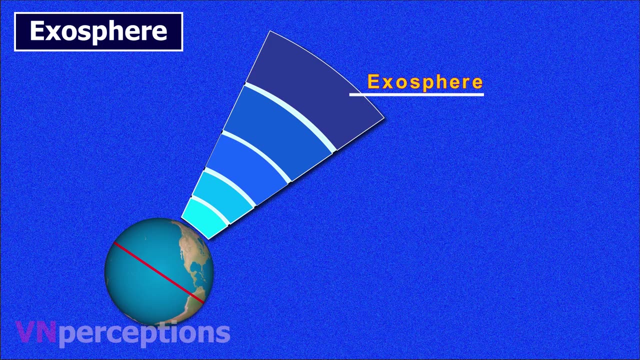 At the bottom of the thermosphere is the mesopause, the boundary between the thermosphere and the mesosphere. below Then comes the exosphere. The exosphere is the uppermost layer, where the atmosphere thins out and merges with interplanetary space. 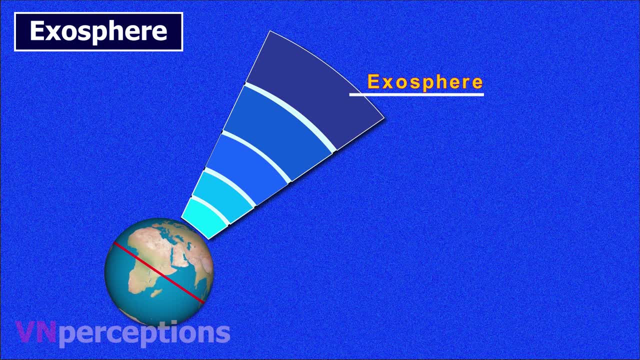 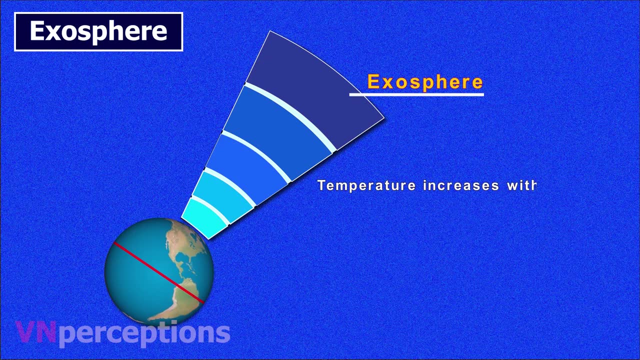 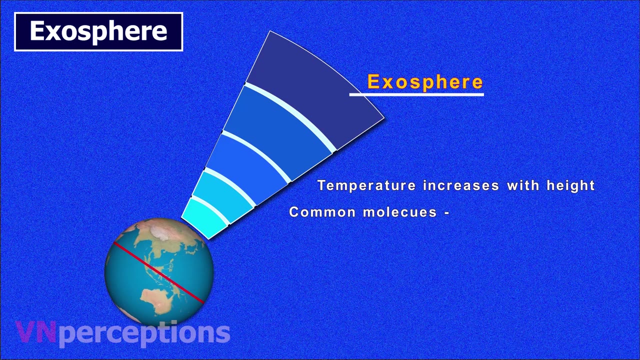 It lies between 500 to 10,000 kilometers above the Earth. In this layer, temperature increases with height. The most common molecules within Earth's exosphere are those of the lightest atmospheric gases. Hydrogen is present throughout the exosphere, with some helium, carbon dioxide and atomic. 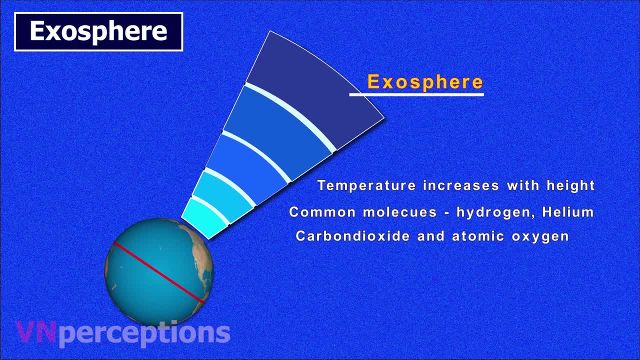 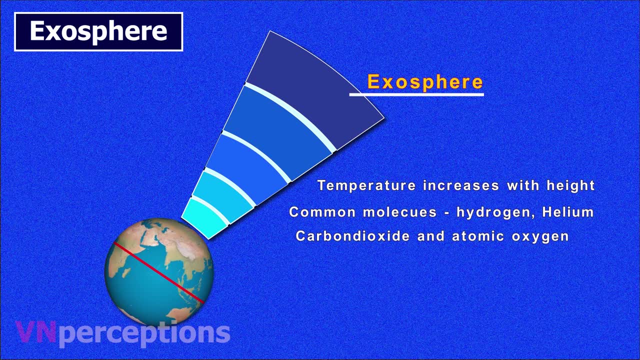 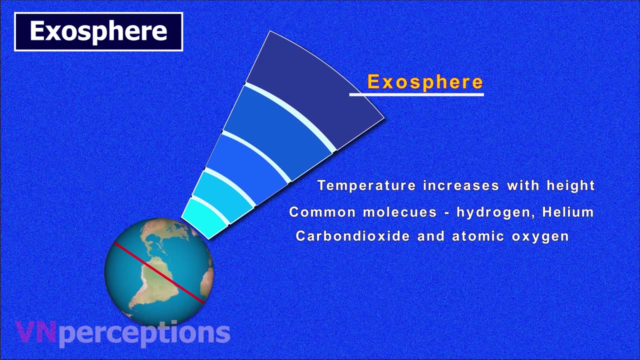 oxygen near its base, Because it can be hard to define the boundary between the exosphere and outer space. the exosphere may be considered a part of interplanetary or outer space. It is located directly above the thermosphere. Very little is known about it. 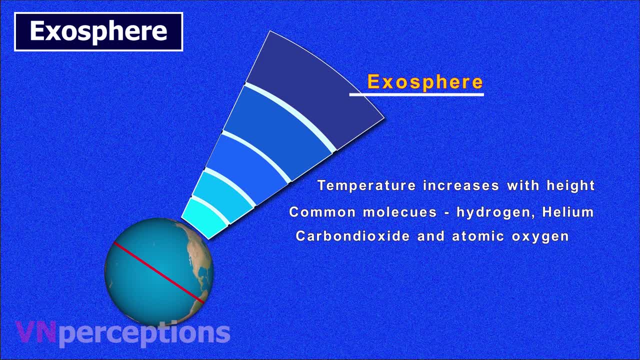 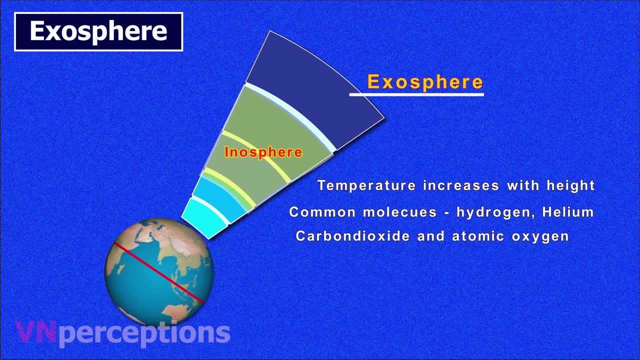 The exosphere is located directly above the thermosphere. Human information is not known about it due to lack of research. The ionosphere is the ionized part of the earth's atmosphere. The ionosphere is located between 60 and 1000 kilometers above the mesopause. 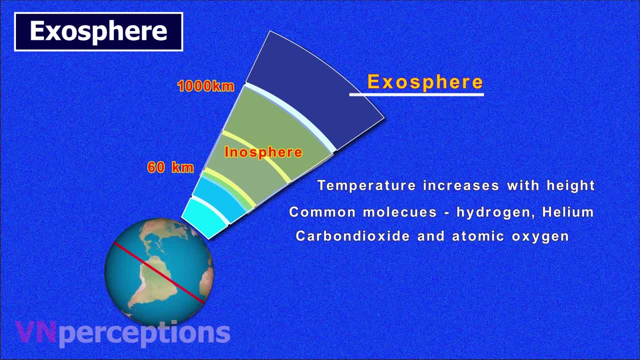 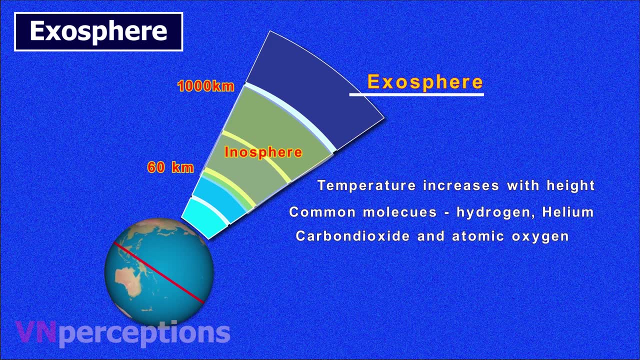 The ionosphere is not a distinct layer like others mentioned above. Instead, the ionosphere is a series of regions in parts of the mesosphere and thermosphere where high energy radiations- from mass wondering over energy flows, depending on current time- are observed and could be dangerously fragile. 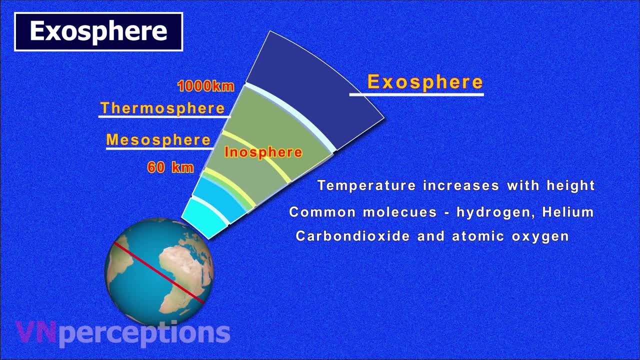 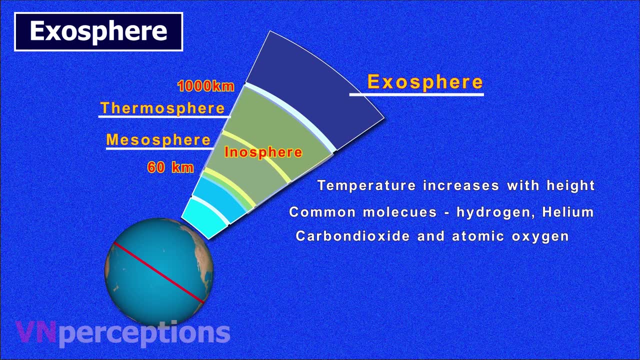 The ionosphere lies between 600 and 1000 kilometers above the mesopause. the sun has knocked electrons loose from their parent atoms and molecules. The electrically charged atoms and molecules that are formed in this way are called ions, giving the ionosphere. 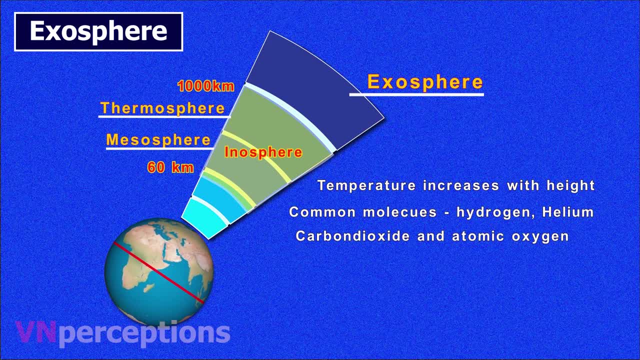 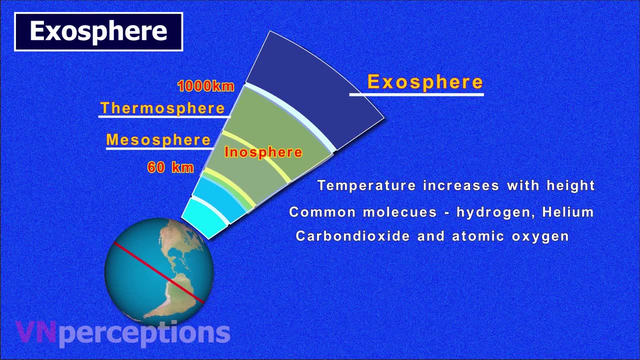 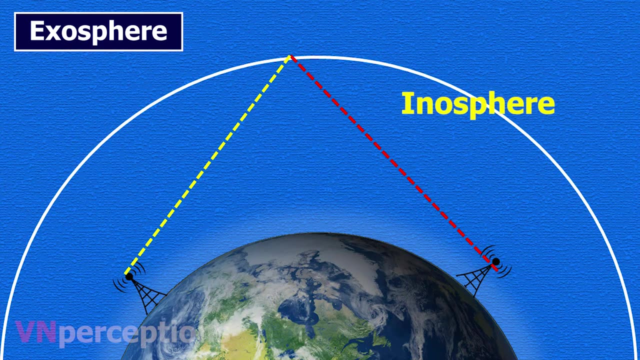 its name and endowing this region with some special properties. It contains electrically charged particles known as ions, and hence it is known as ionosphere. Radio waves transmitted from the earth are reflected back to the earth by this layer. It contains electrically charged ions, which